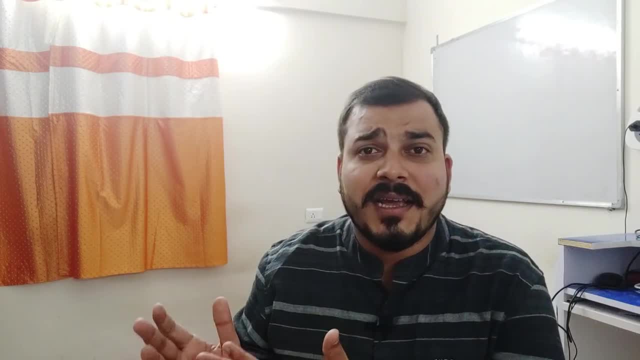 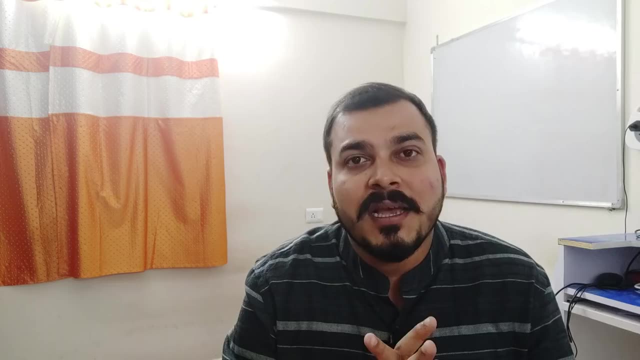 know what I have to do. I usually follow a particular life cycle and I know that in each and every stage what I have to do. So I'm going to mention you some of the tricks, some of the techniques which will actually help you to become good in exploratory data analysis. Yes, to become an expert, it will 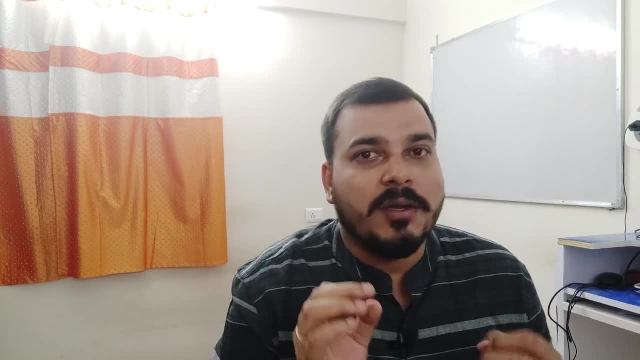 definitely take time and you need to know how to do it. So I'm going to mention you some of the tricks which will actually help you to become an expert. it will definitely take time and you need to practice a lot of things. So what do I do in terms of exploratory data analysis? So, as soon as I get 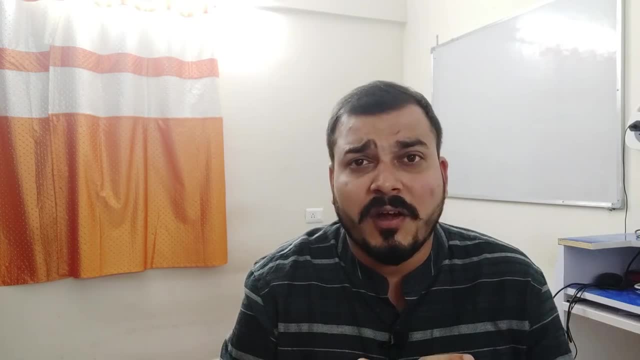 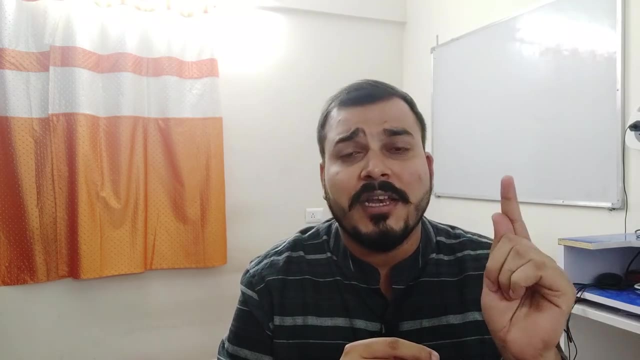 the data set right, let it be. let it be having millions of records, let it be having any number of columns. The first thing. I just go with the life cycle of a data science project. I always tell you that after you get your data, okay, then you have to do the feature engineering part Now. 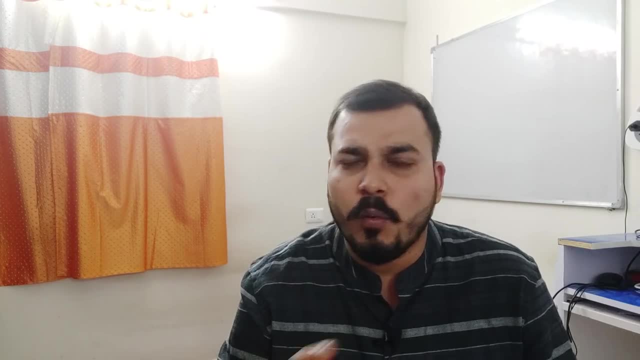 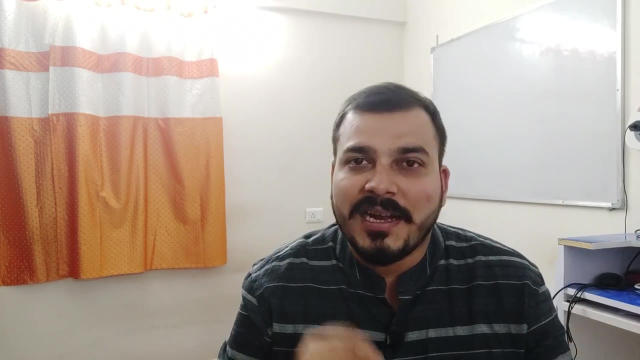 in feature engineering part. first of all, I go and handle the missing data whatsoever. I have basically, you know, defined that thing in my mind itself as soon as I get the data set. So I'm going to go and handle the missing values. So I'll go and check how the missing values are there And 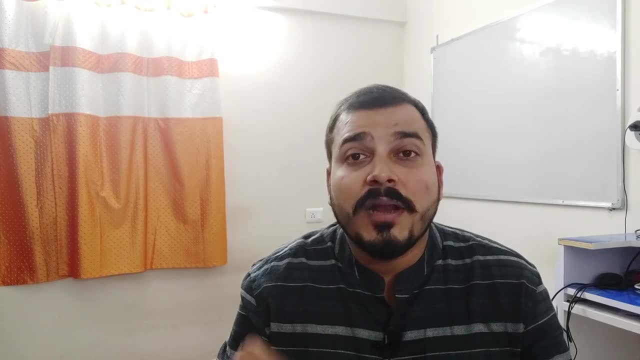 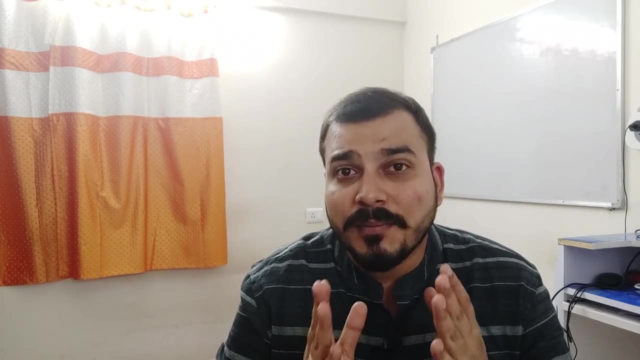 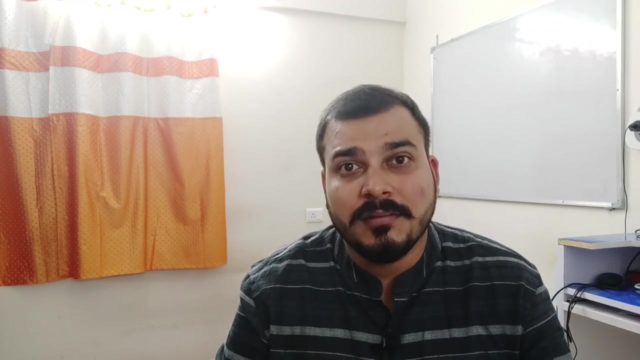 again, you have to be good at Python. You have to be good at Pandas and NumPy library. It is must OK. Apart from this, you also have to be good at some statistical visualization libraries like Seaborn and Matplotlib. So this four are must OK: NumPy, Pandas, Seaborn and Matplotlib. Four things. 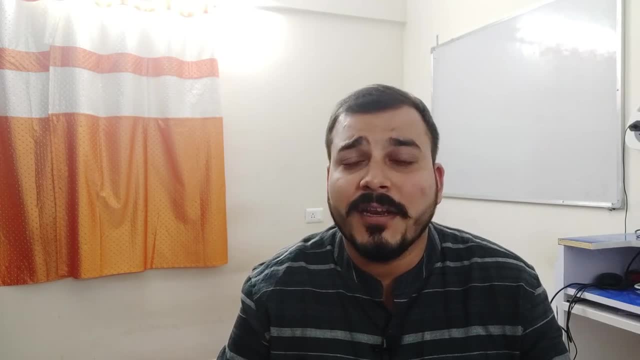 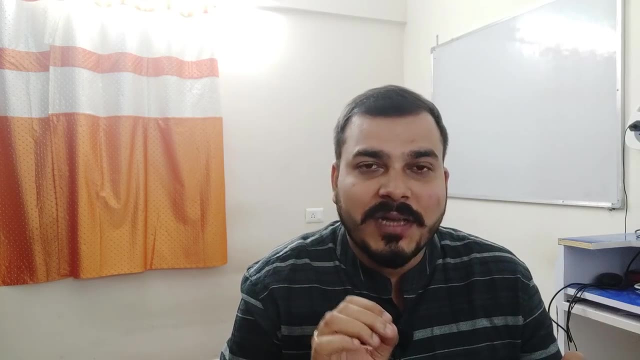 If you are good at this things, definitely no one can stop you in becoming a very good- you know- expert in exploratory data analysis. So, first of all, what I do is that I handle the missing values. I make sure that there are no missing values in the data set, And again over there I'll be. 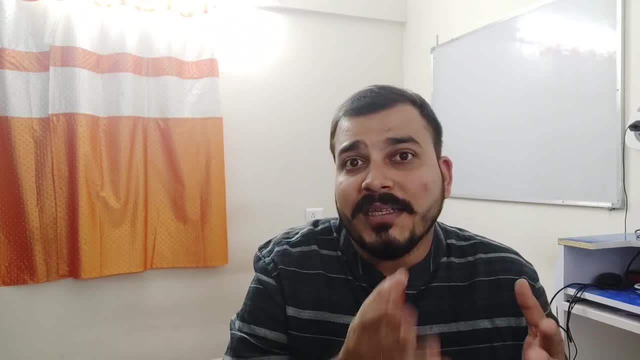 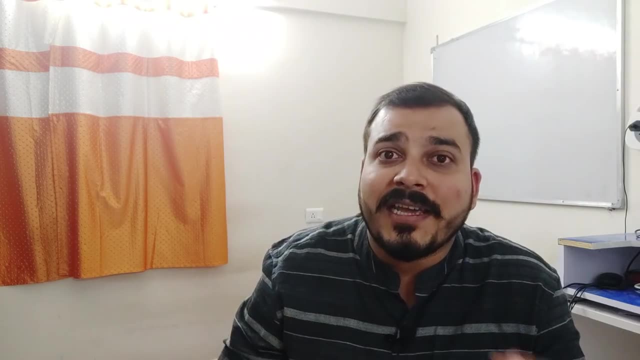 including Seaborn and Matplotlib, both because Seaborn helps us to apply statistical analysis on the data. Suppose, if I want to handle the data missing, data itself, Right, Based on the distribution of the data, I can select mean median mode or end of the distribution, and there are 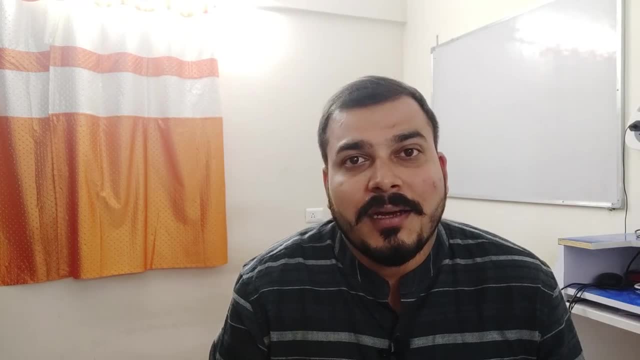 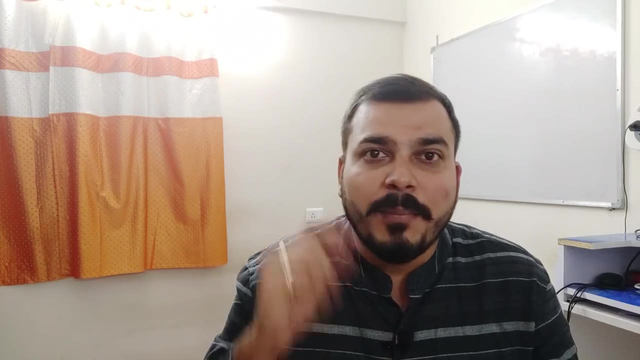 no missing values. Now one more thing I would like to add. Right Initially, a person who's getting shifted to data science, he may not know all the methods. So how do you, where do you go and refer all those things? The best thing is that you go and refer Kaggle kernels. OK, All the different. 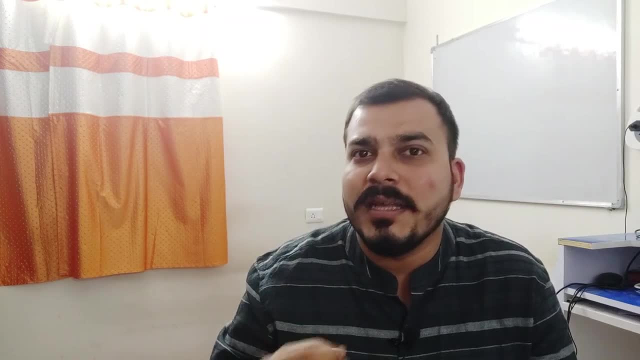 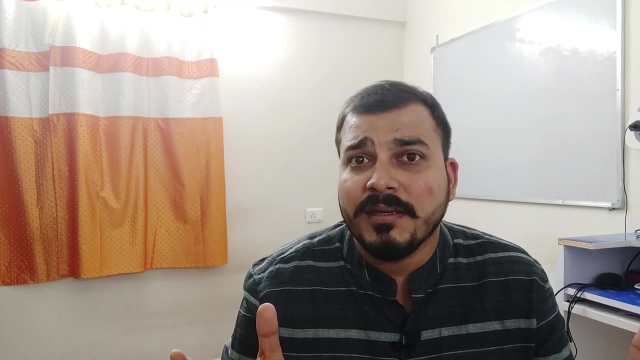 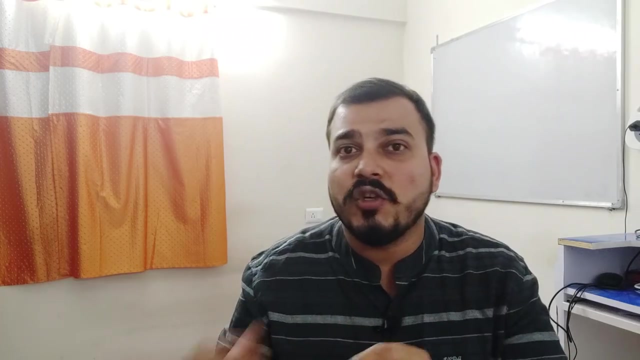 types of technique used by people, used by Kaggle rankers, are given over there. They provide that kernel: No read blocks from medium towards data science Right. Many blogs have been created over there. Yes, You can definitely use it, because the different techniques- and again I'm telling you there are no fixed techniques- Tomorrow you may 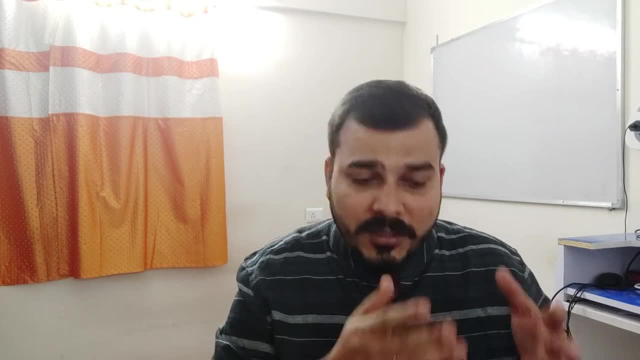 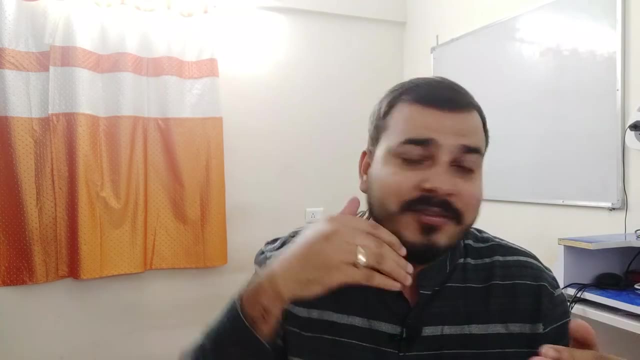 come up with a different technique of handling the missing value, Right, But you should know at least some of the techniques, how to handle the missing values itself and how I have gained that. I've seen a lot of examples. I explore a lot of examples how they are basically handling missing. 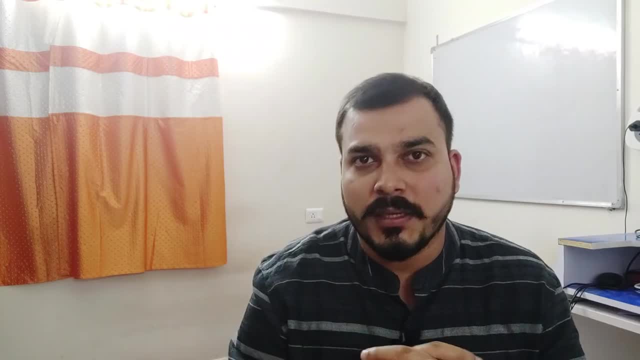 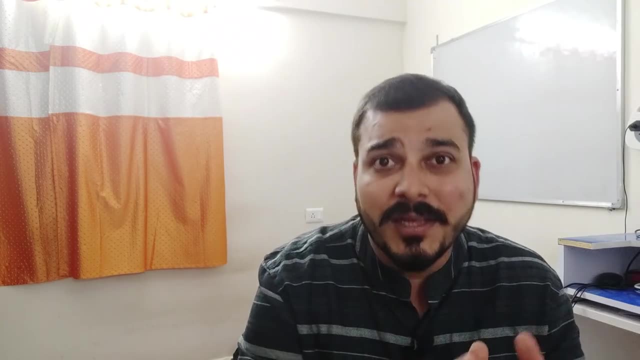 values, How is the accuracy are impacted with the help of that and many more things. So always remember this is how you have to learn, guys, because if you want to become an expert in some thing, you have to give. And again, it is openly available in the Internet. You can definitely use. 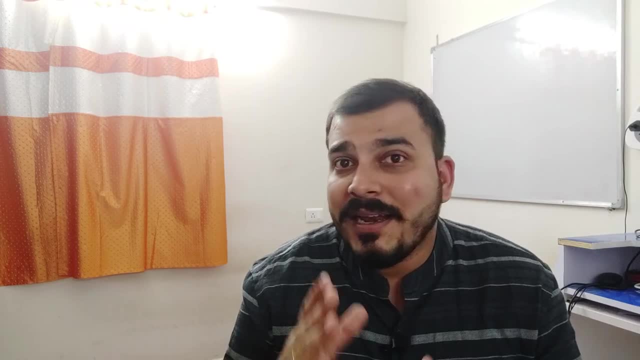 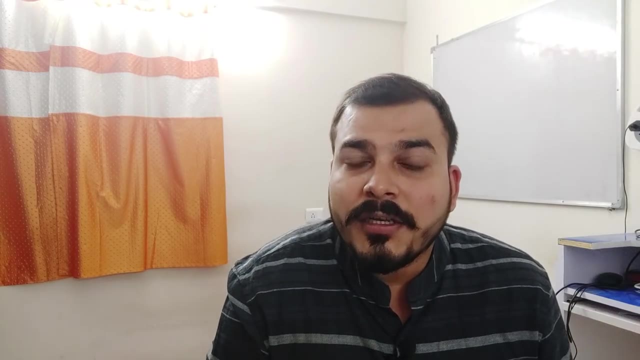 it for your work purpose, Right, This is one of the thing. And again, after you go and handle your feature engineering, Suppose I go and I'm trying to handle the missing values. I've explored all the techniques. OK, I know by myself around seven to eight techniques of handling missing values. 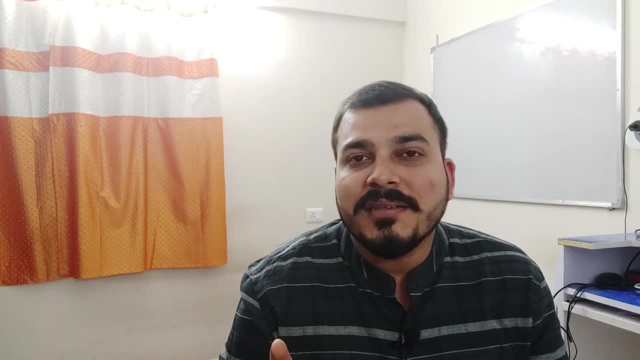 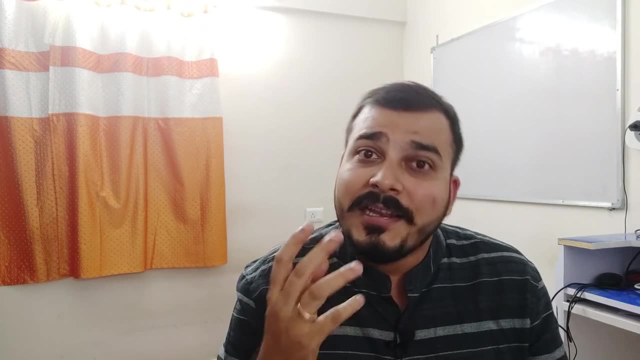 And this is through exploring through different Kaggle kernels. The second way is that suppose now missing values is fixed. Now you go and try to handle the category feature. OK, Because this is also part of feature engineering. Then again, there is not only one technique to handle category. 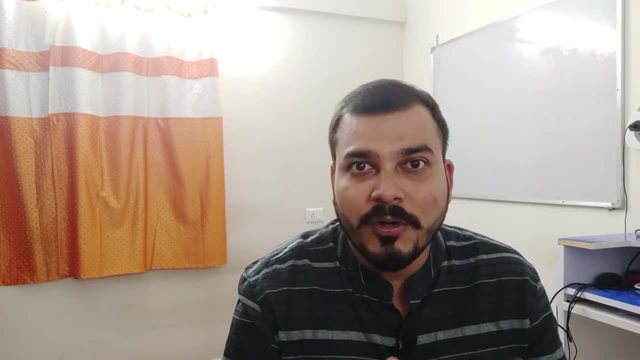 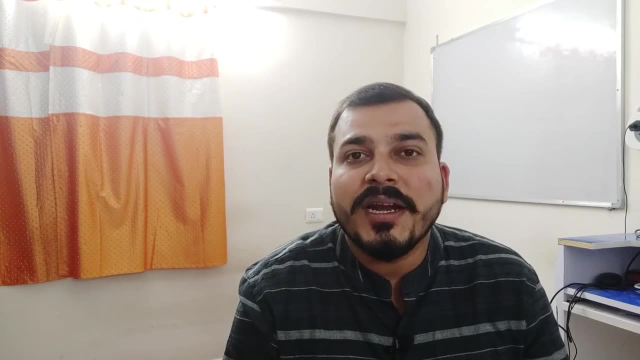 features. There are multiple techniques. There are eight to nine techniques still now known And again there are scientists who are actually using some different techniques also and they're exploring with that and they're trying to find out whether they are able to get good accuracy. 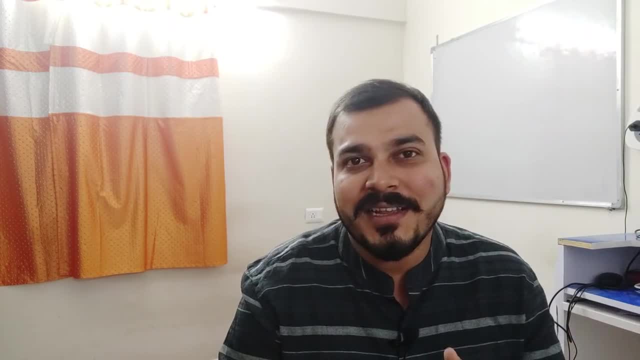 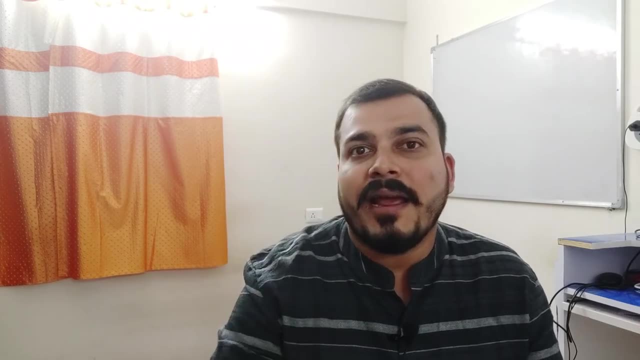 And again, how do you, how do you find out? how many different techniques are there? Research, You know, go and find from the blogs. go and see Kaggle kernels, See how people have got. You know they have Kaggle rankers who will be putting all the information in different different blogs. 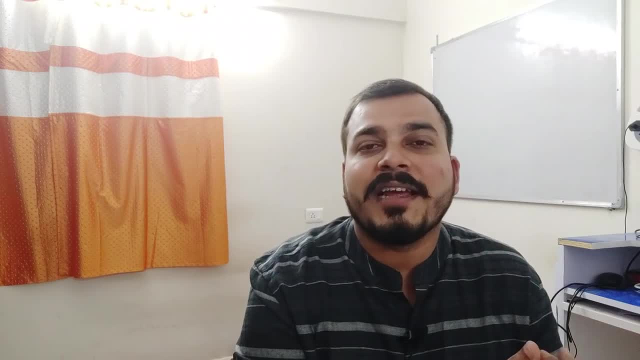 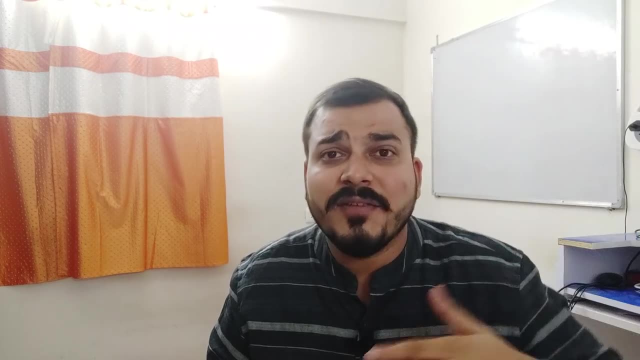 Go and search it. How did they handle those scenarios? How did they handle Kaggle feature, Suppose I have? I have something like a postcode, OK, And they will be. each and every pin code or the postcode will be having will be considered as a different category feature. How do you handle that? 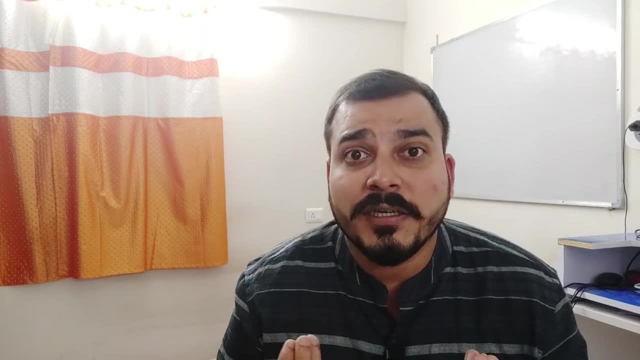 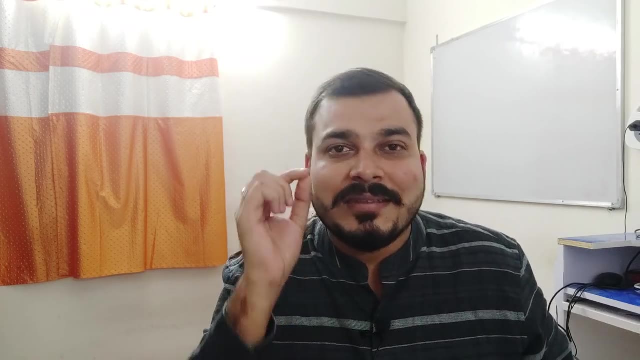 Right, And this is how you should always be: having that curiosity And what, what, what, if, like, if you have, if you know nine to 10 different ways, automatically you'll be thinking of the 11th way by yourself. Trust me about that, because you'll be having so much of knowledge to. 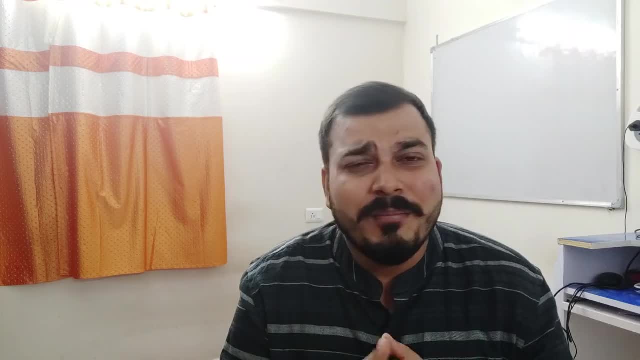 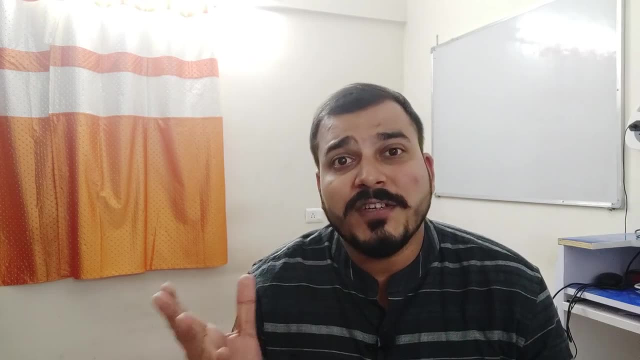 handle those kind of scenarios. Now this is how you have to do again for imbalanced and balanced data. You have to try to find out different ways. That should be your main aim. OK, Each and every scenario. Now, when I go to feature selection, the main thing is that should I consider each and every? 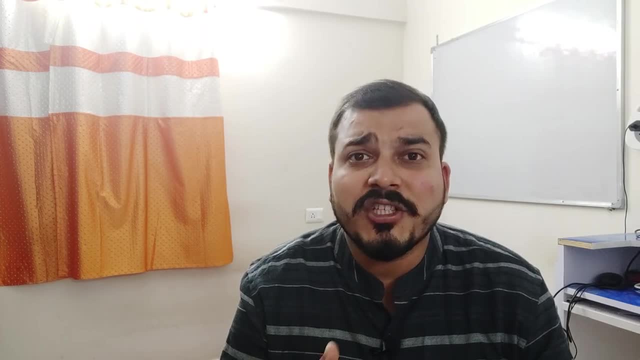 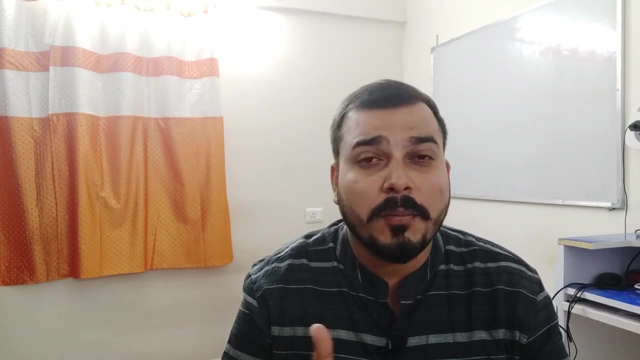 feature. How can I do that? There are a lot of techniques, again by correlation, Pearson correlation, Spearman, rank correlation, Right. Apart from that, apart from correlation, again they have forward propagation, backward propagation and many more Right. So just try to find out what are the. 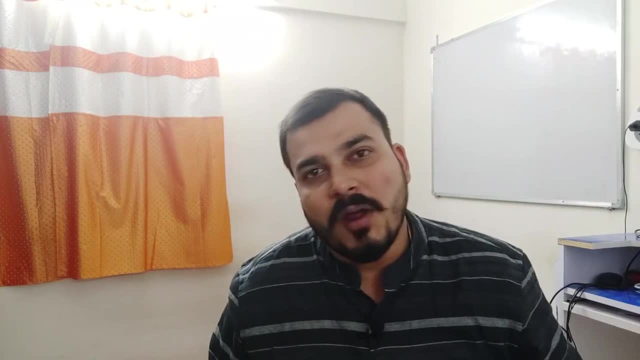 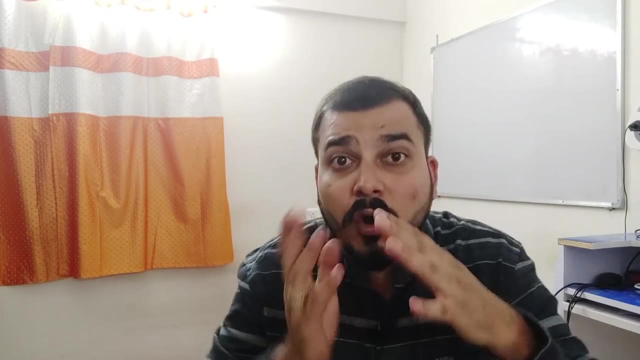 best and after practicing for some n number of problems, Right, You will automatically come to know that. OK, this technique will get properly applied to this kind of data set because you already have that particular experience. That is the major thing that you need to understand, OK, 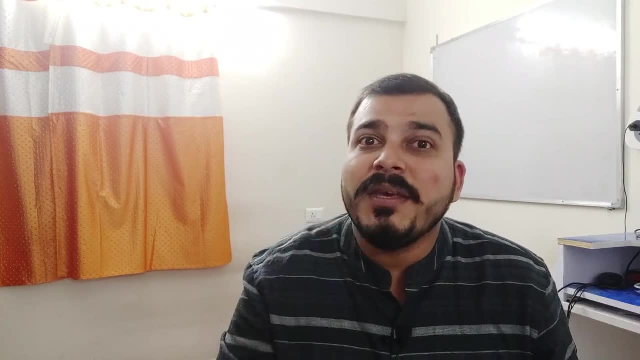 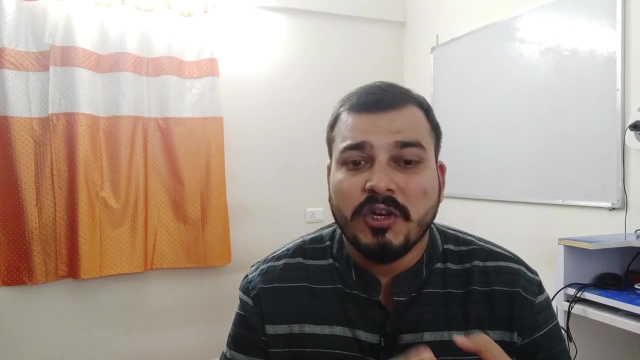 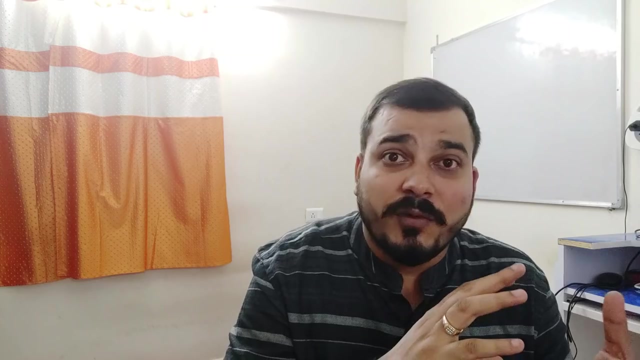 And one more point that I would like to mention. guys, please be very, very good at NumPy Pandas. you know Matplotlib Seaborn. This should be, must. You know, Seaborn, most of the libraries over there have features like this plot, joint plot. You know, this plot actually helps you to create a different. 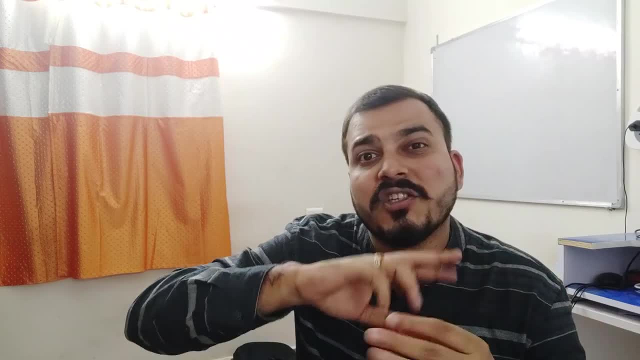 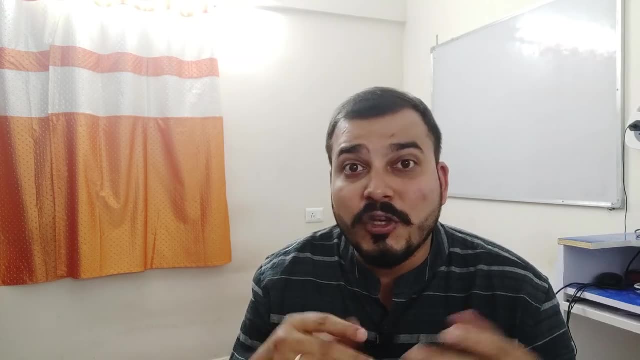 and you also have something like pair plot. This plot actually helps you to create the histograms. along with that, you'll be able to create a kernel density estimator and many more things. Right, You have pair plot for the univariate analysis. You have different plot, you have joint plot and many. 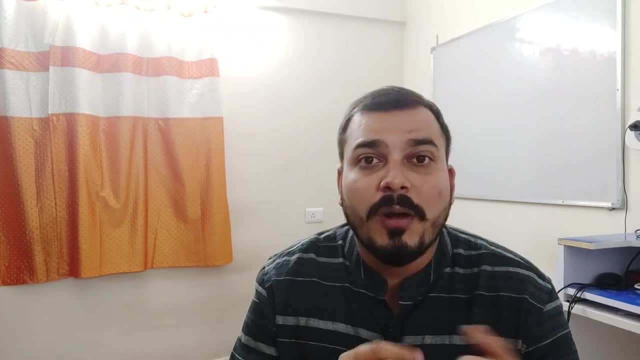 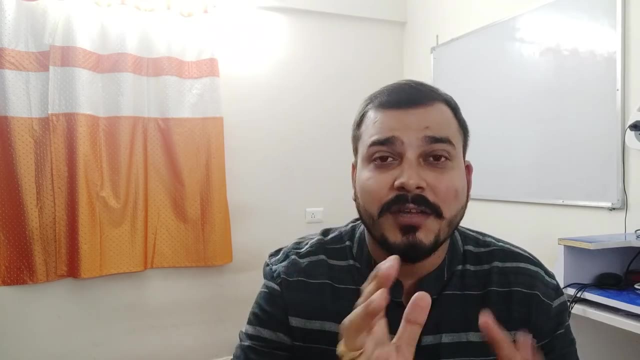 more things. You have to explore them. And there is also something called as count plot based on category features. They are different types of plots. Again, don't worry, I'll be uploading those videos, as I told you that I'll be uploading all the videos in Python. I'm going to include Pandas and always remember. 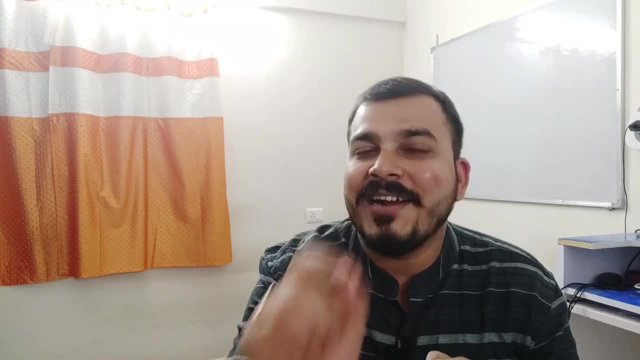 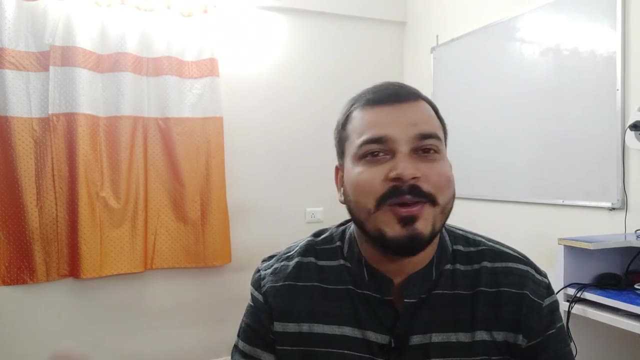 Pandas is must, guys, because you will be able to read any kind of data sources you want. If you know Pandas, I think most of your problem statements is getting solved because you're able to load the data set and they are a lot of complicated data sets also. OK, Suppose in that data set you have 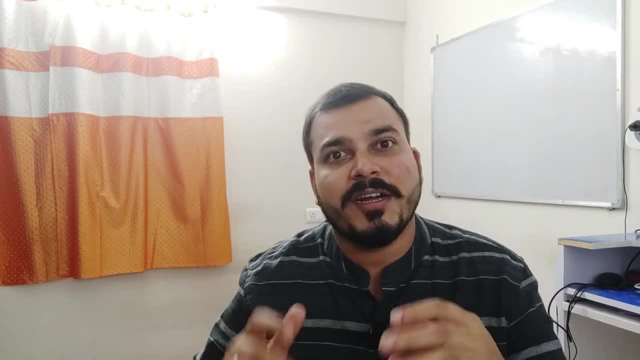 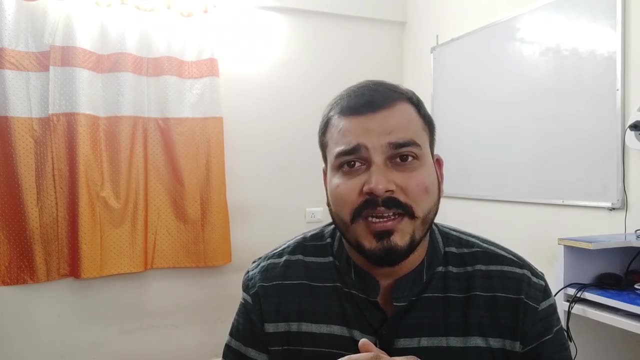 comma separated. Suppose it is a CSV file. You have comma separated. You have tab separated. You have a new line separated. Various things can come into a particular data set. That basically means that data set is not clean, Right? So you should be very, very sure about and. 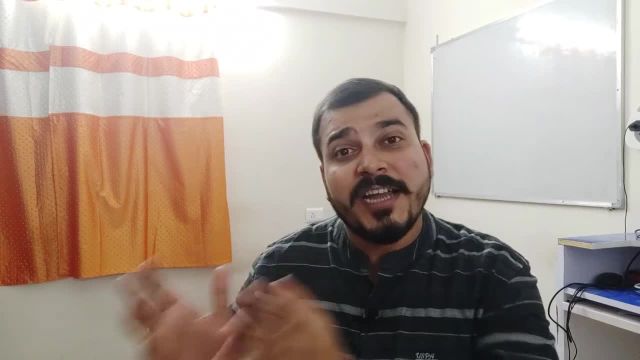 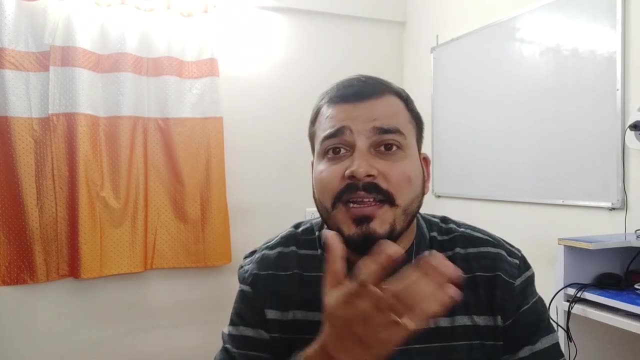 you should be able to find out different, different techniques. Different, different techniques should be your main concern. Let me just give you one example, If I just consider handling the category features, like you know, many of them knows one hot encoding. Many of them knows label encoding One. 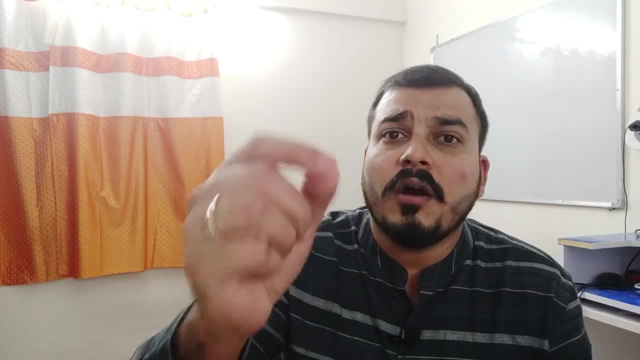 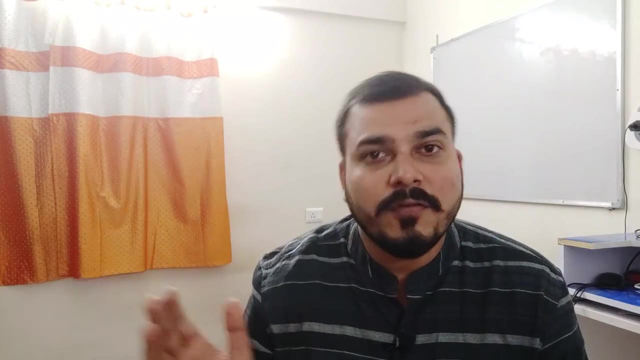 hot encoding is for nominal variables. Label encoding is for ordinal variables. What if? And you know that in one hot encoding, If I Divide these categories, it will be creating that many number of columns. Right, And what is the disadvantage in this? If I have a category feature, if I have thousand columns, that thousand? 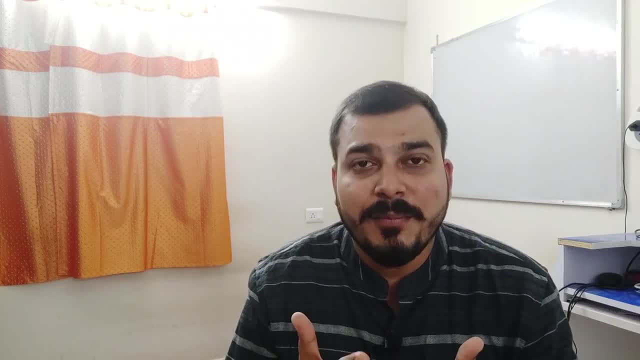 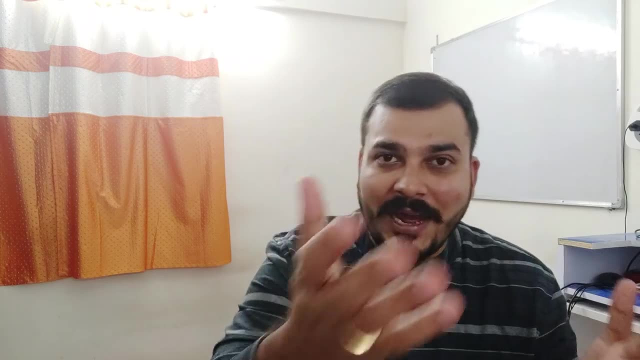 categories, that will, in turn, create thousand columns Right, Which is very, very bad. Yes, So now you should explore what are the different ways. How do you do that? Yes, I know I've already uploaded videos on how to handle category features if they are multiple categories, And that is. 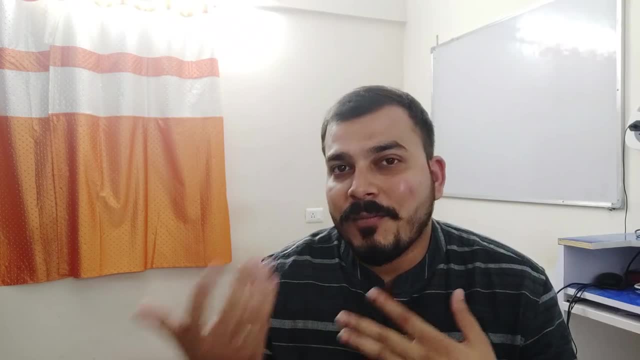 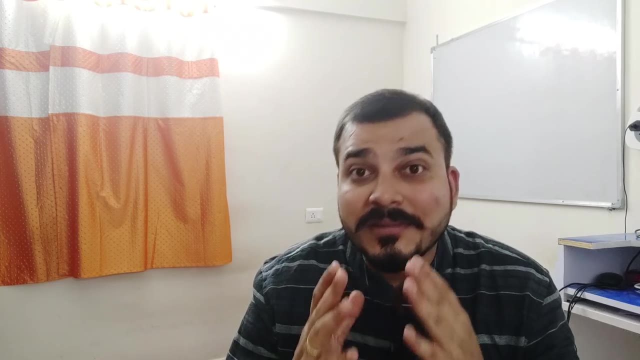 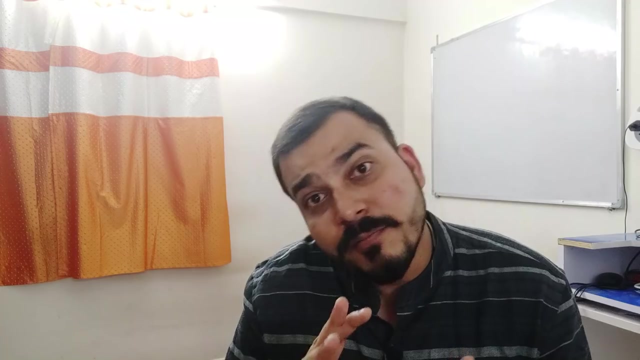 through different, different reference. I also got from the references of blogs, from the reference of references of Kaggle kernels and many more things. So this must- again, you should always have the curiosity to learn more how I can do this thing with different, something with a different. 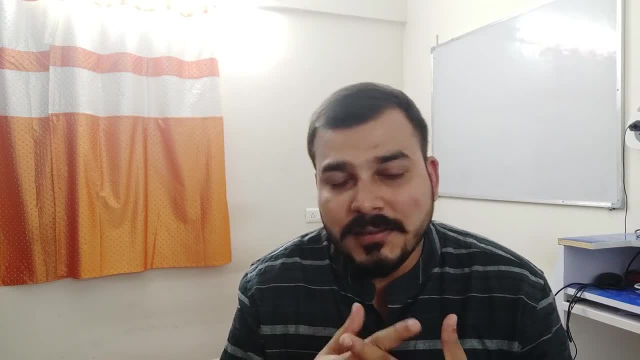 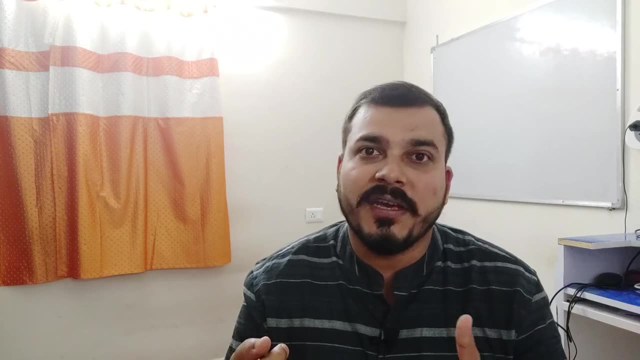 approach. This is the problem that is basically happening in this, And that is all, guys. You just have to follow that path. Try to find out many ways, Try to solve a use case with all the ways and see how your accuracy of the model is getting impacted, Because in the later stages, whenever you 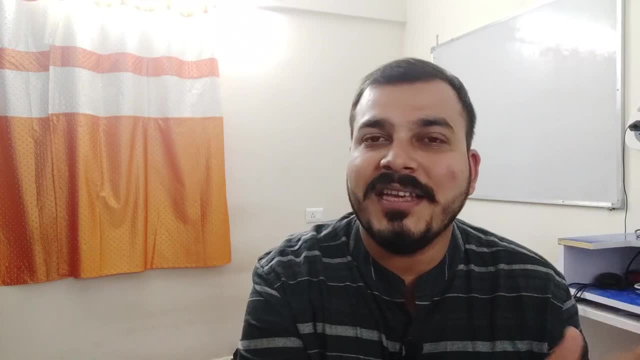 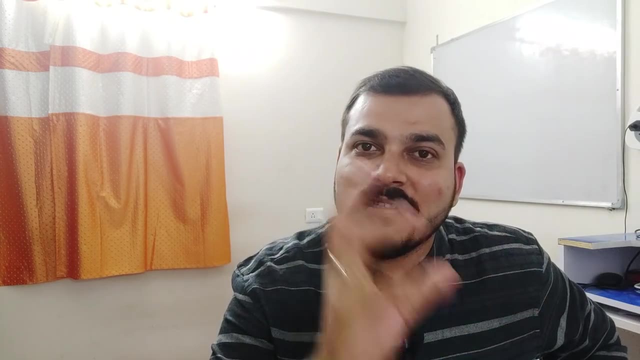 get a new use case? definitely. you'll know that. what kind of techniques I have to have used for handling the missing values, because I have the data set like this. Make sure that you do that statistical analysis with the help of Seaborn also, because the Seaborn gives you the visualization of.